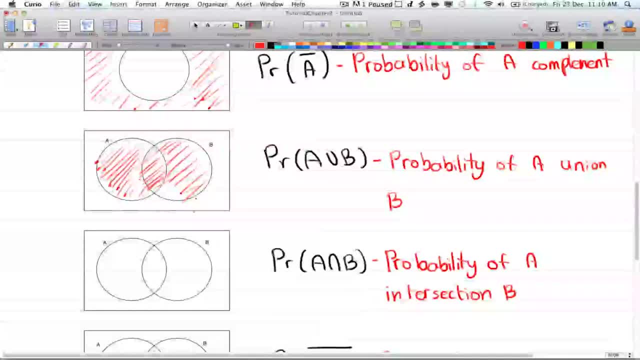 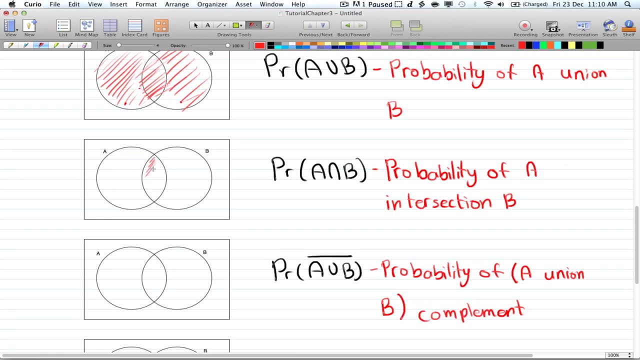 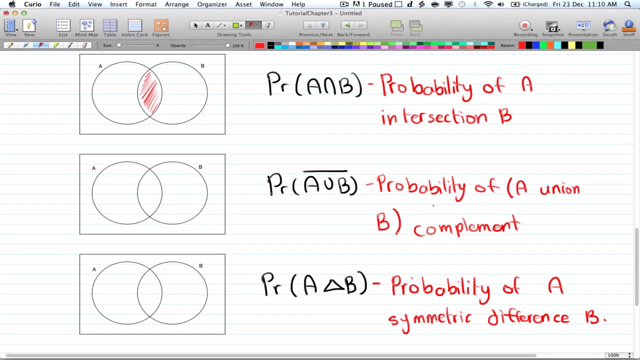 and the part in between their intersection. The probability of A intersection B is just what A and B have in common, so it's just this part here And the probability of A union B complement is everything outside A and B, So everything outside both circles. 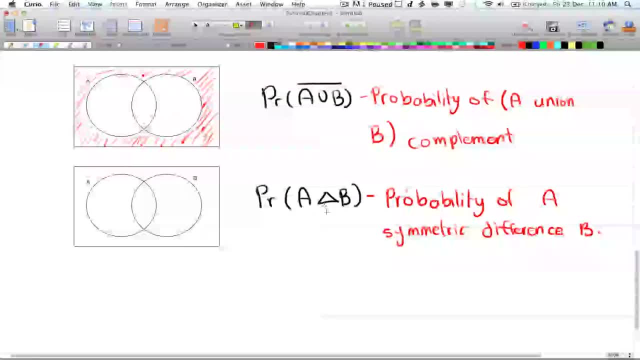 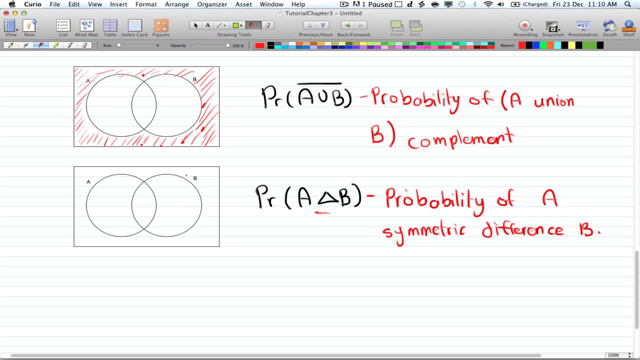 Alright, and the probability of A symmetric difference- B- and there's a sign for symmetric difference- is everything inside A and B, excluding their intersection. So it's everything inside A and B, but not their intersection. So this part here does not count. 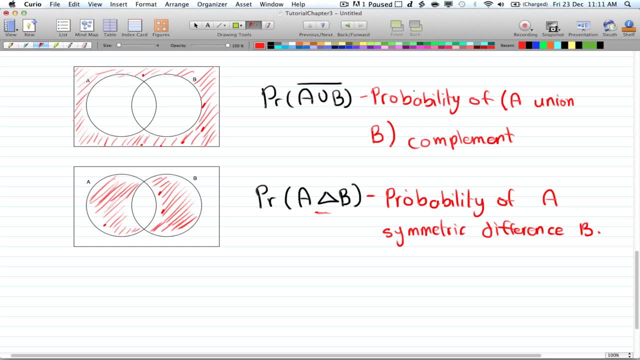 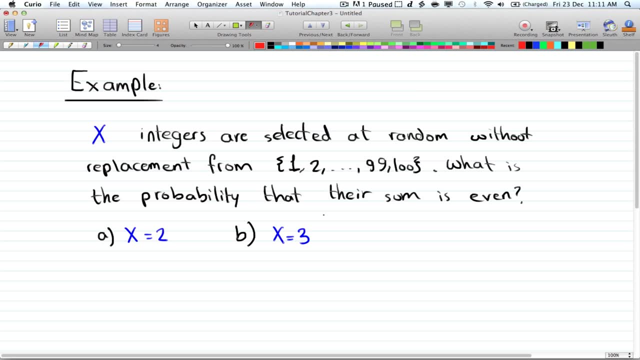 Alright, so that was some basic names for probability. Alright, so let's take a look at an example. So let's say, x integers are selected at random, without replacement. So you take one integer, you cannot use it again, And the range is from 1 to 100. 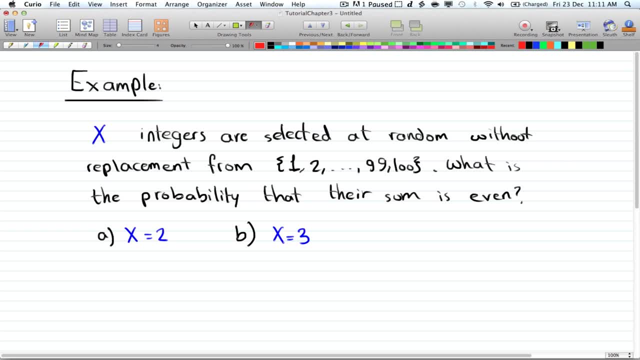 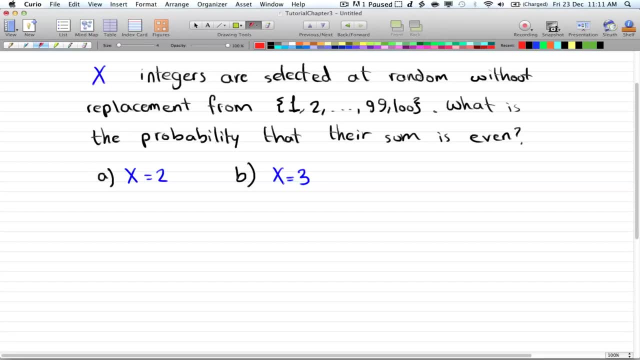 Now, what is the probability that their sum is even? And for the first part, part A, we're going to take- x is 2, so two integers are selected at random, Alright, so the way to go about this is if you have a sample space. 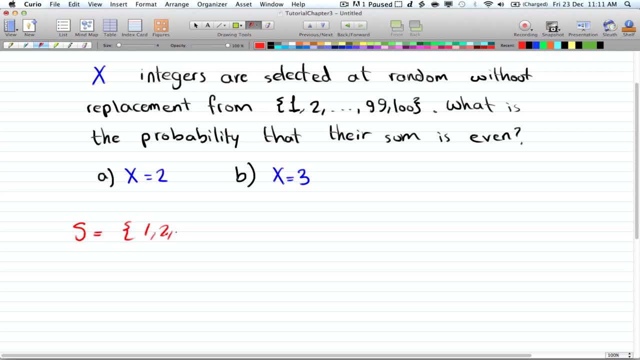 so the sample space is 1,, 2,, 3,, 4,, all the way to 100.. And you have to take two numbers from there. So the probability of the sample space or like the, yeah, the probability of the sample space. 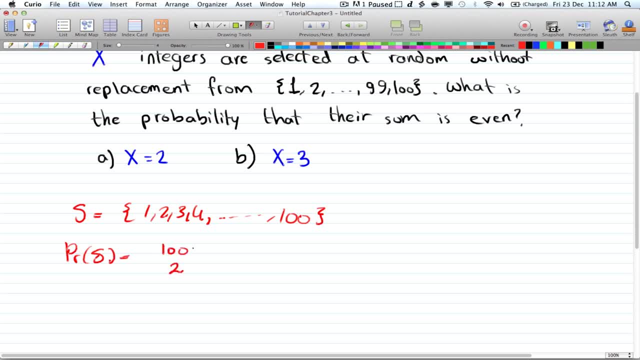 is equal to 100 choose 2, because you're taking two integers only, And that is equal to. let me hit into the calculator: 100 choose 2 is 4,950.. Okay, So if you take two integers, there are two ways of getting an even sum. 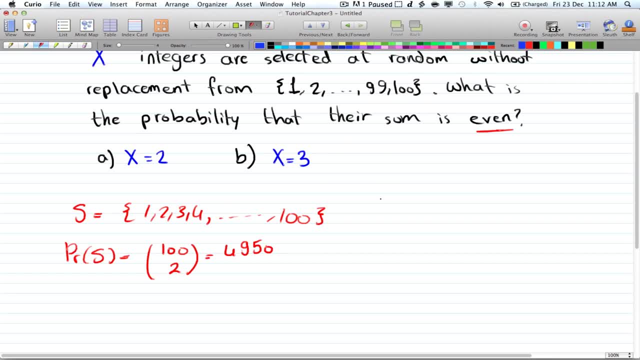 One is. if so, two ways of getting even. Either x and y are even, that's called integer 1, x and integer 2 is y, So they're both even, Or x and y are both odd. So that's the two ways of getting an even sum. 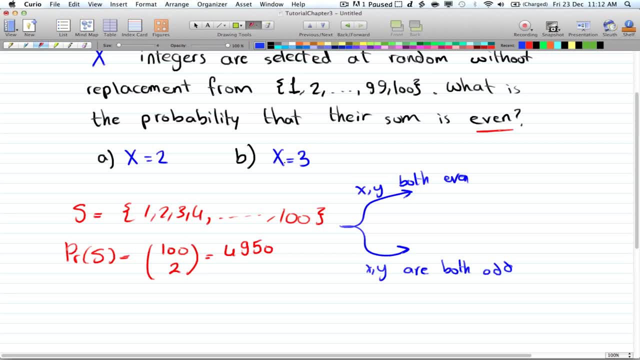 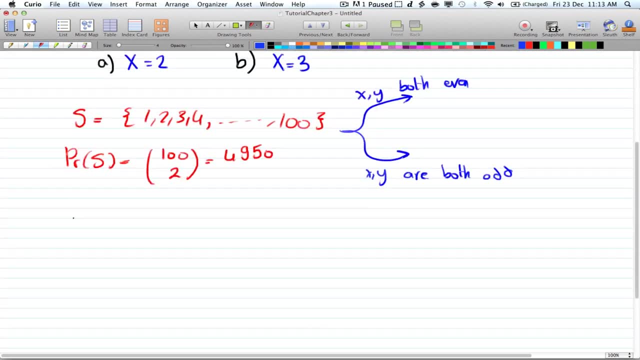 Or the two ways of getting two integers to be even, Or the sum of two integers to be even. Alright, so here you have. a is equal to x comma y, where x plus y equals an even number. So that's like the sample space for it. 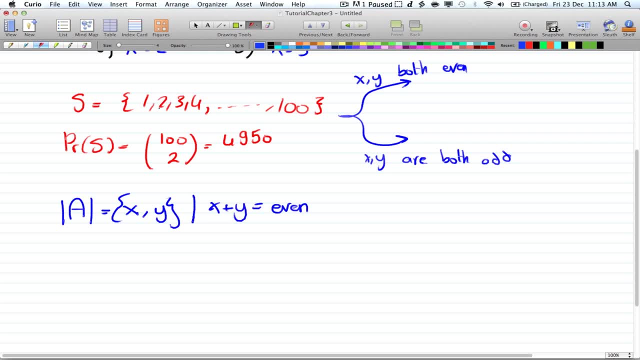 Alright. so if you have to pick an even number out of 100, from 1 to 100, there are 50 even numbers and 50 odd numbers. So if you want both to be even, then that is equal to. 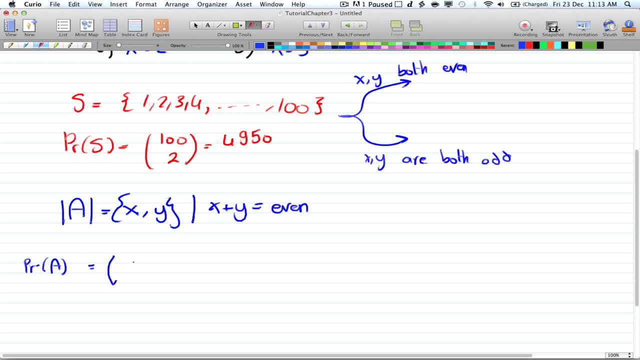 so the probability of a is equal to 50 choose 2.. So that's the probability for even numbers. So here that is even. Both are even, And the probability of picking two odd numbers will be 50 choose 2.. So here both are odd. 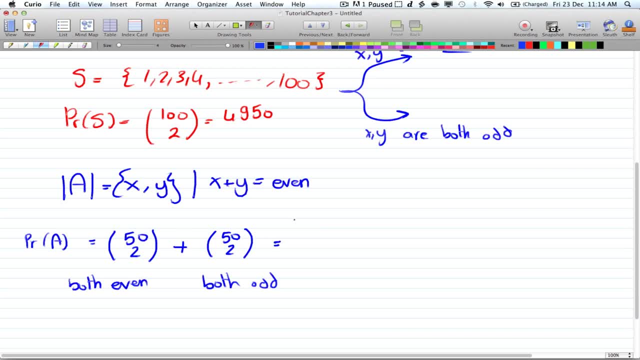 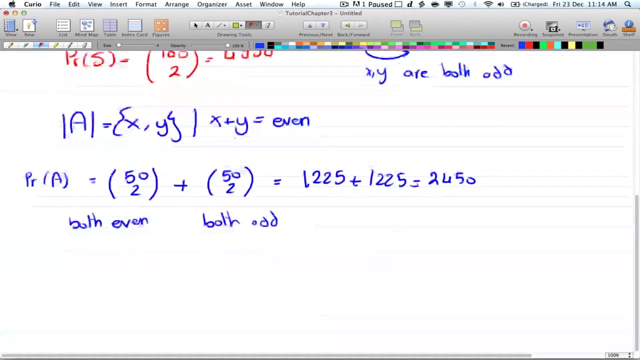 And if you just sum them up, you get the probability of a, which is equal to 50. choose 2,, that is 1,225.. Plus 1,225,, which is equal to 2,450.. And now to get the actual probability of a. 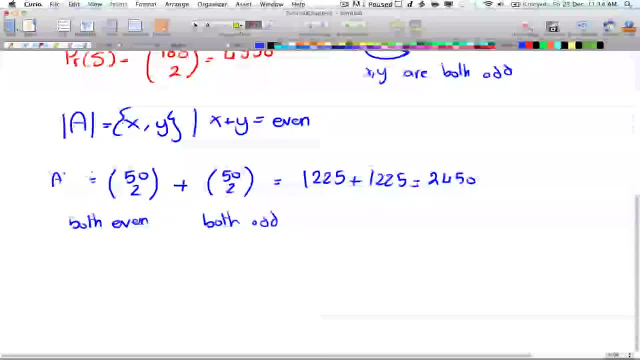 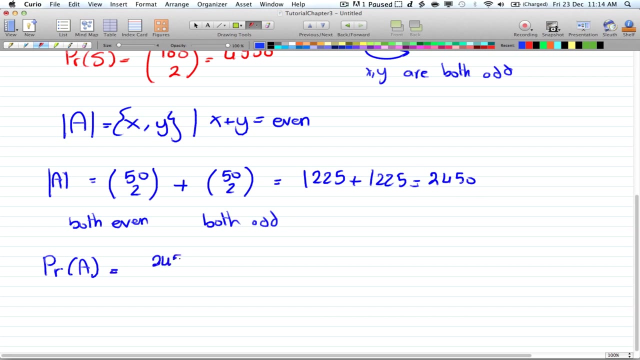 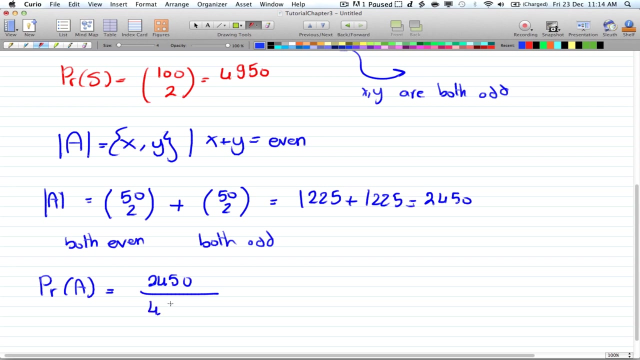 sorry, this is the number in a, So the number of possibilities in a, So the probability of a is equal to 2,450, which is the number of possibilities in a divided by 4,950.. So 4,950.. 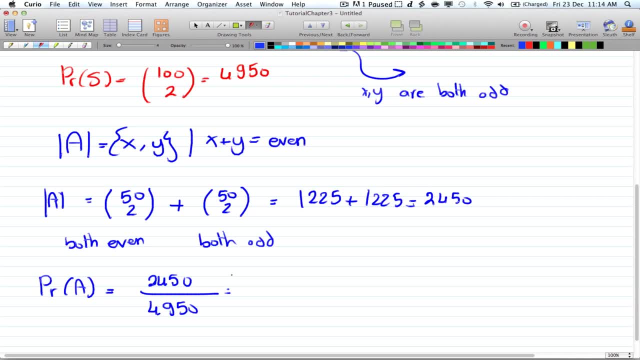 And that is equal to 0.49.. And one thing to check when you're doing probability: if you're getting a number greater than 1, then you're definitely doing something wrong, Because the probability is always smaller than 1,.